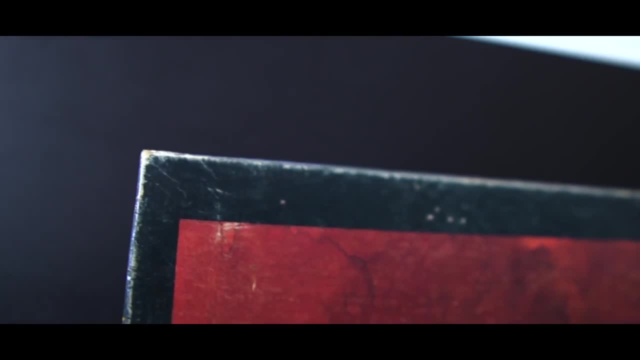 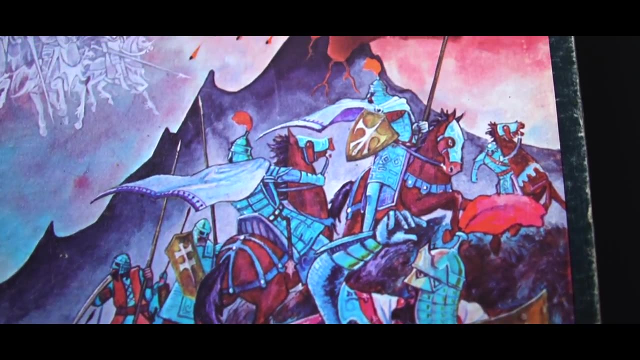 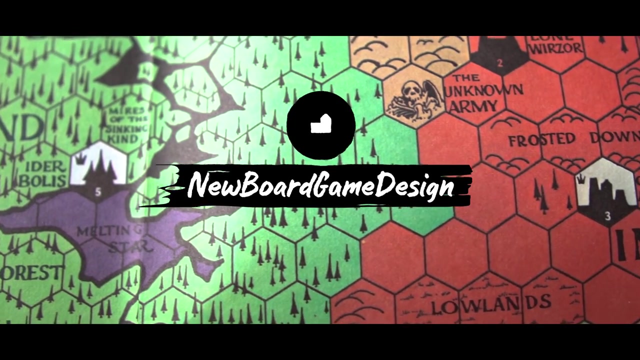 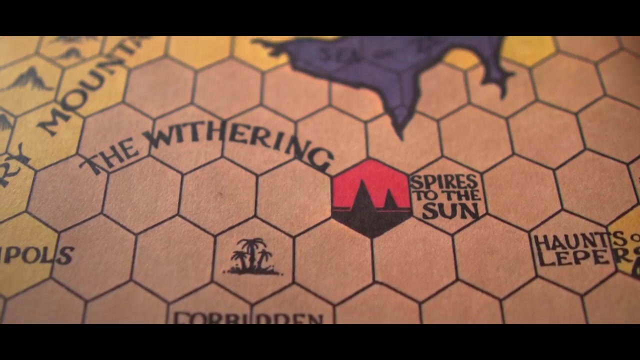 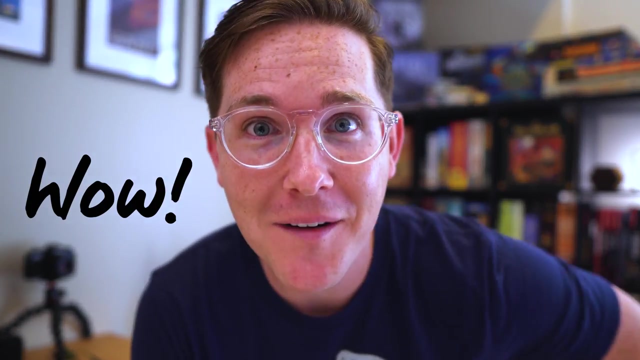 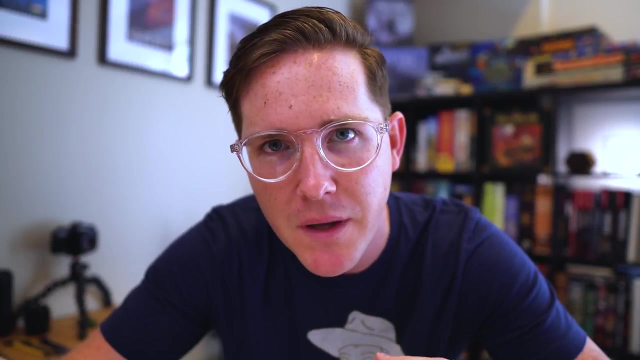 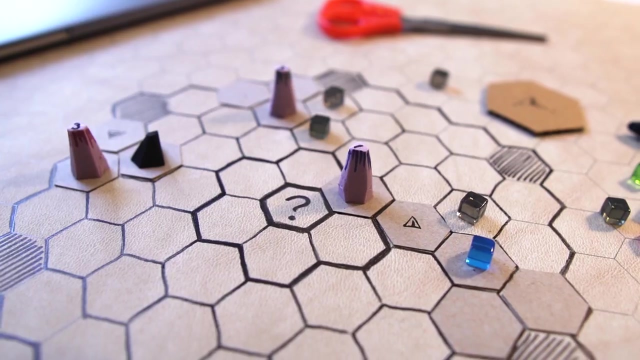 Okay, okay, Wow. Thank you so much for the engagement on the channel so far. I started this channel to celebrate the design process of developing and designing games, and you are helping me do that. Thank you so much. This is the second video talking about my exploration game that. 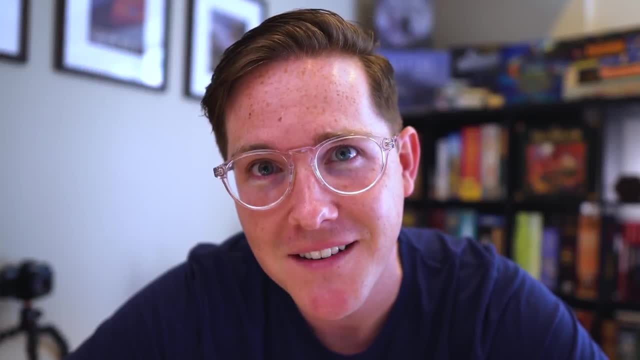 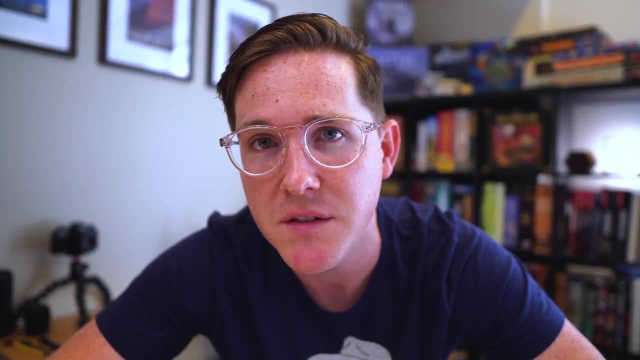 I'm designing and I'd argue this is the fun part. I want to show you the multiple examples of the game mechanisms that I've come up with so far. Again, I'm definitely early in the stages of the design process for this game, but brainstorming the actions components, 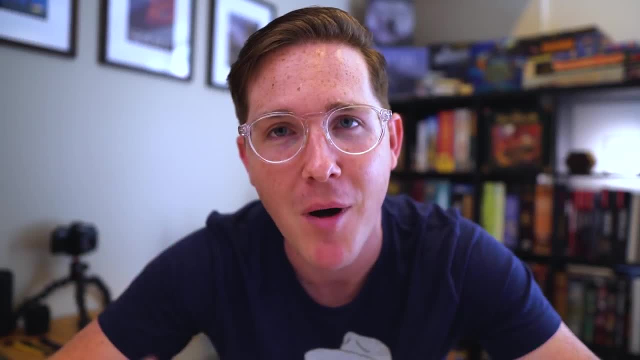 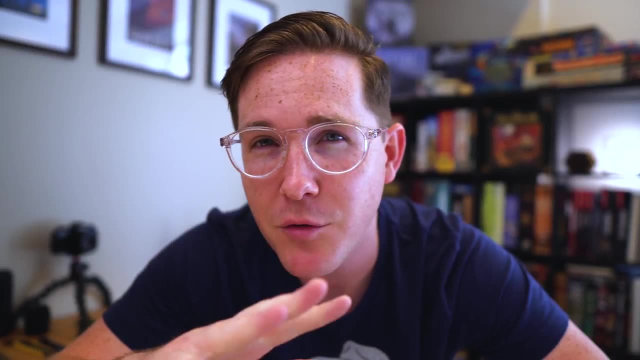 and any combination between the two is my favorite part, Because, to me, this is the point where the possibilities feel endless and my creativity is sparked the most. I get to throw as many game mechanisms, cards, components, tokens, board layout, everything out on the 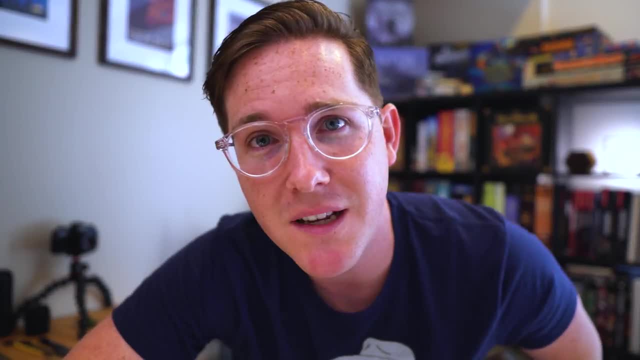 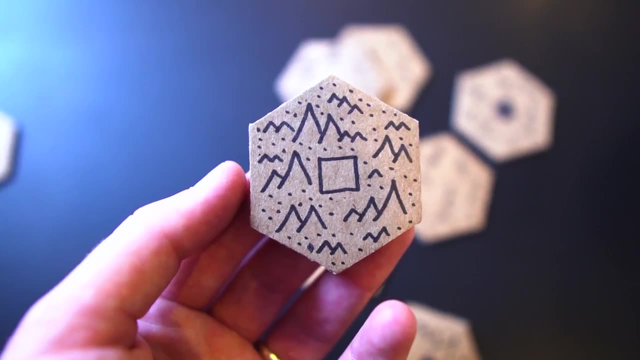 table and pick from the best. Also, this is my favorite part, because I tend to design and create prototypes in tandem. If I have an idea about a Hex tile, well, I want to make a Hex tile to try it out. If I have an idea about the board, well, I want to see it on the table. In this video, I'll 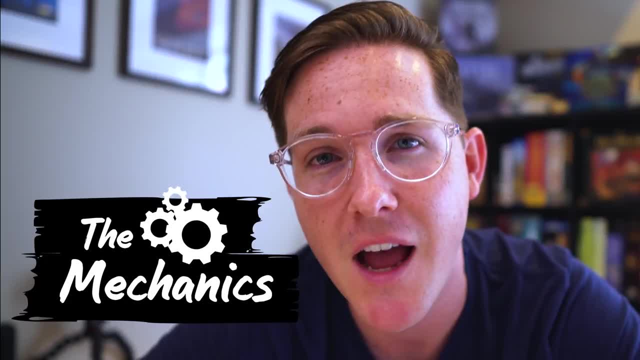 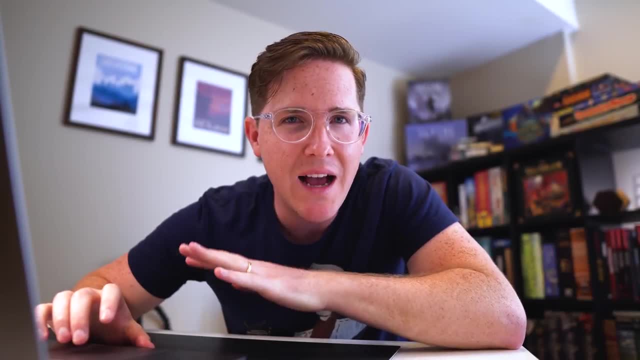 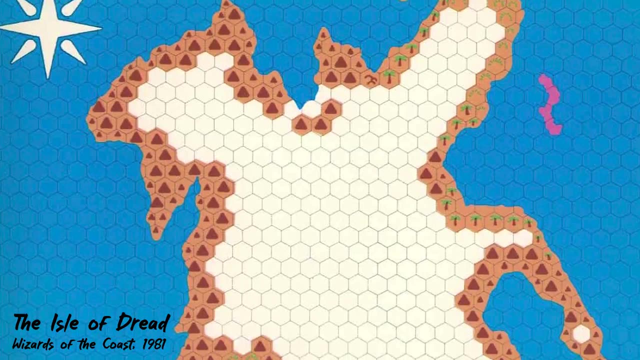 be showing you ideas about mechanisms and the rough prototypes I have so far. Thanks for watching. Have you seen those classic D&D Hex tile open world maps- I think they're called Hex crawl maps- where it's just an ocean of blank Hex tiles? They tempt your curiosity because you 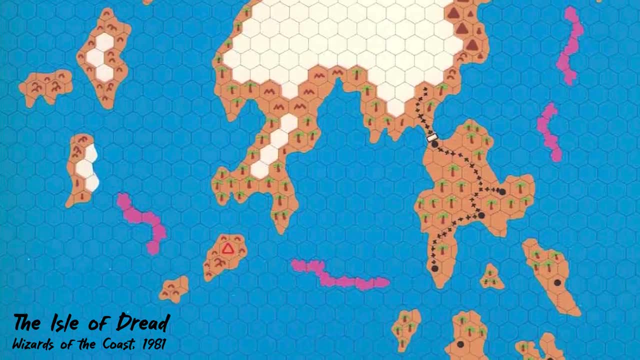 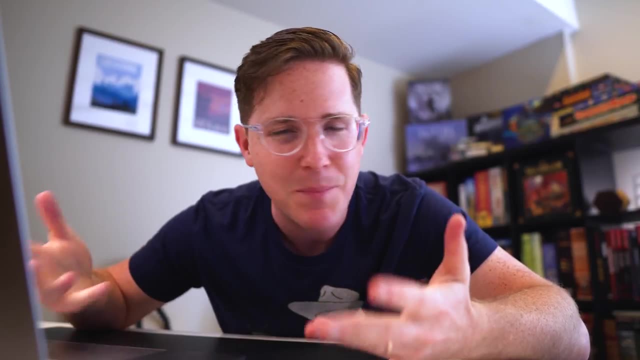 look at all the Hex tiles, and you think to yourself, wow, look at all the possibilities in front of me. They tempt your curiosity even by showing you a map of empty spots, of empty spaces, because you think, well, look at all the locations I can go to. I wonder. 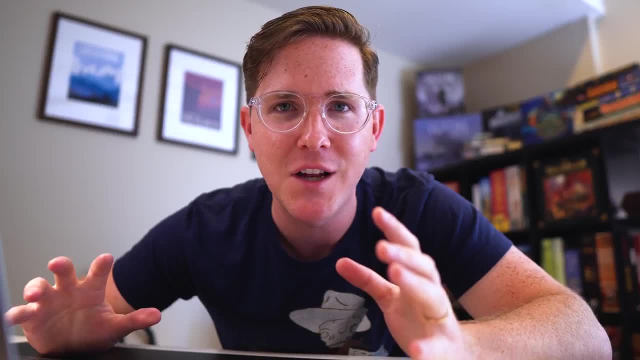 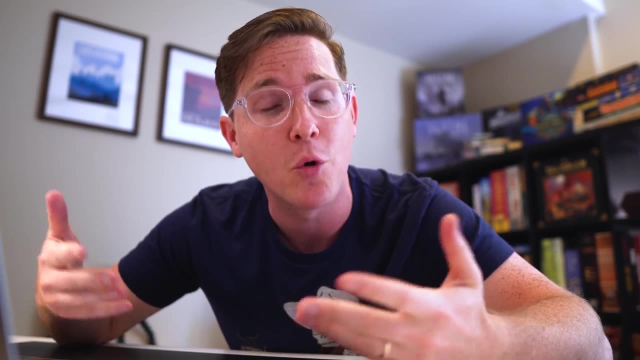 what's in store for us on each space. You can't help but start imagining what challenges or obstacles or rewards the DM or the Adventure Guide have in store for you throughout that continent or world to explore. I don't know about you, but whenever I see an open world, 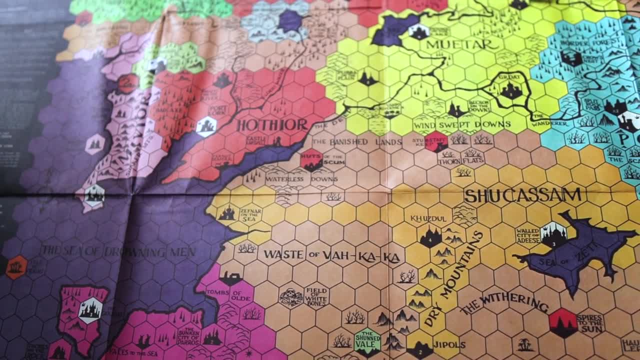 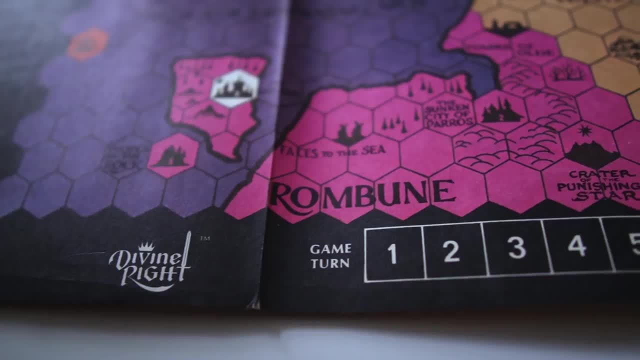 map like that, an expanse of hex tiles, an expanse of open spaces. It's like looking at a map of an amusement park. There's so many things to do in front of me and I really don't know where to start. 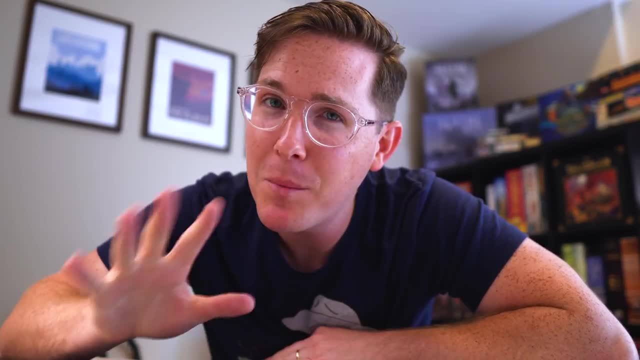 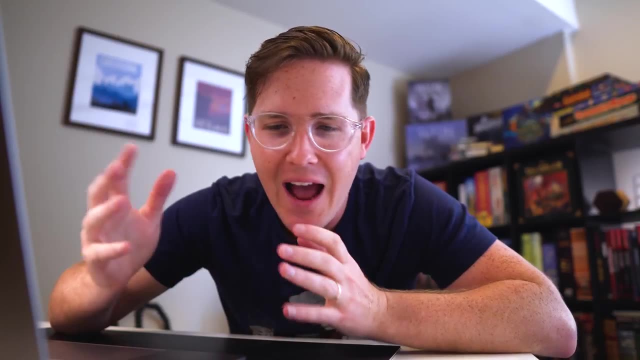 Now, that is a good feeling to create in a board game And I'm aiming for something similar in my game- Maybe not to that scale, but something similar- If your board can make people gasp and chuckle out loud as you lay the board down on the table. 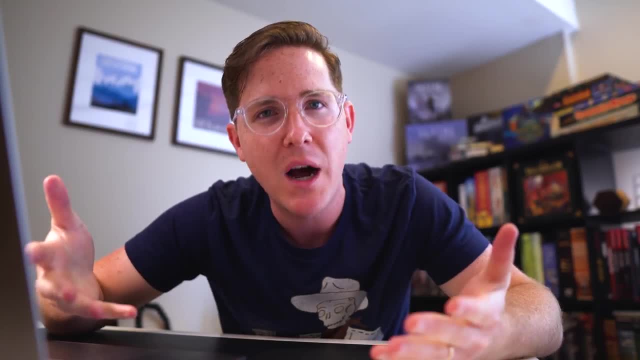 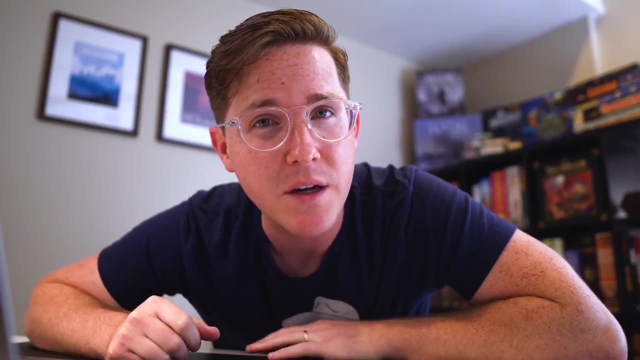 and their minds start racing and they get excited about all the things that they could possibly do in your game. then I think you're doing something right. as a designer. You're heading in the right direction. But now you've gotten your players' hopes up. 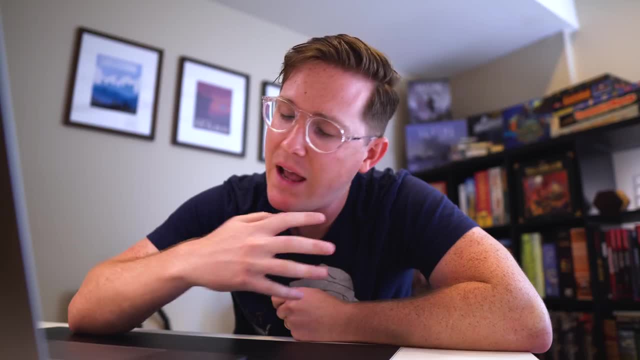 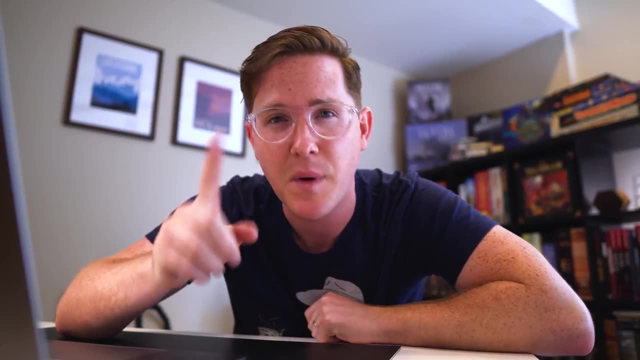 for an adventure that waits, and now you need to deliver a good game. Anyone can throw a ton of hex tiles and open spaces on a board and incite a feeling of awe for an adventure game, but it takes a responsible designer to deliver on that expectation with a solid system of actions. 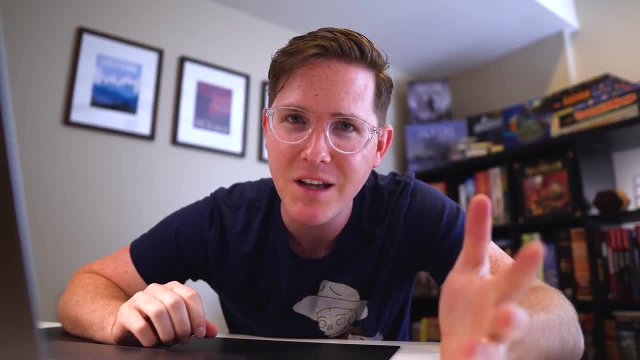 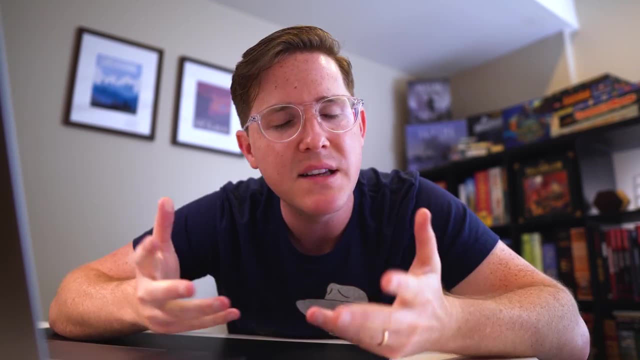 challenges and rewards to make a game fun to play. This makes me think about my favorite games like The Legend of Zelda and The Witcher series, and how it doesn't matter how big your open world map is unless the things that you can do in that world are fun. 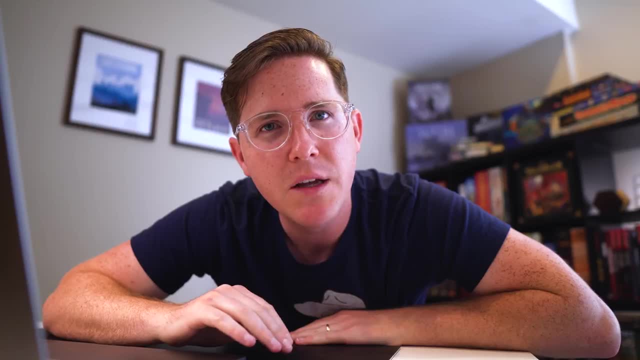 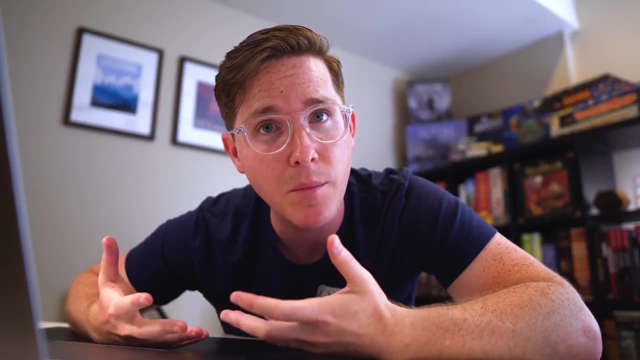 tied together somehow and keep the players coming back to the game to explore more and go deeper. Okay, that was a bit of a rabbit hole, but you get my point. My game is aiming to offer something similar: a healthy helping of exploration. slash adventure. 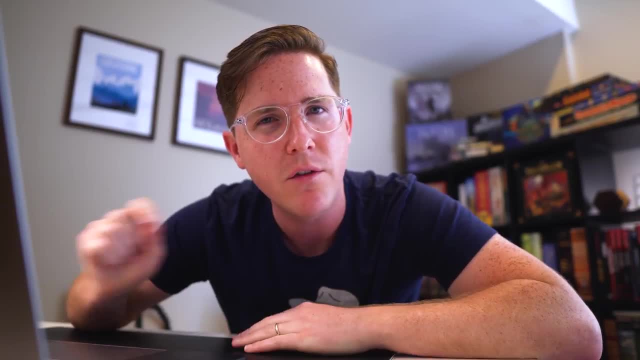 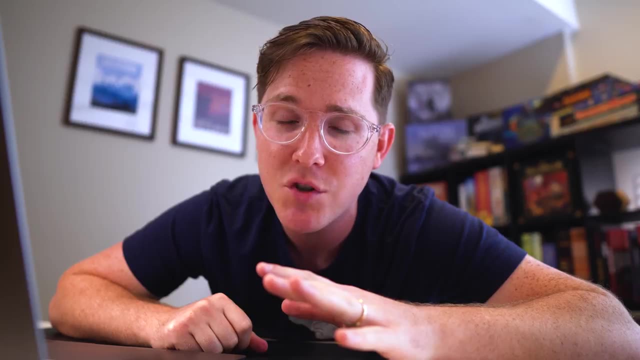 gameplay experience, just with a simpler delivery method and in the form of a board game. Obviously, I would never try to make a board game as immersive as The Witcher 3.. No one's going to have the choice to play a quick hand of Gwent. 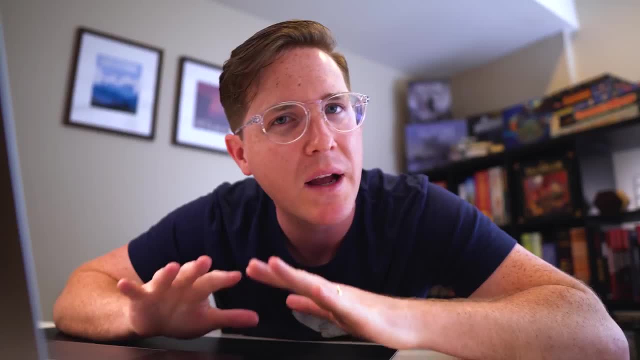 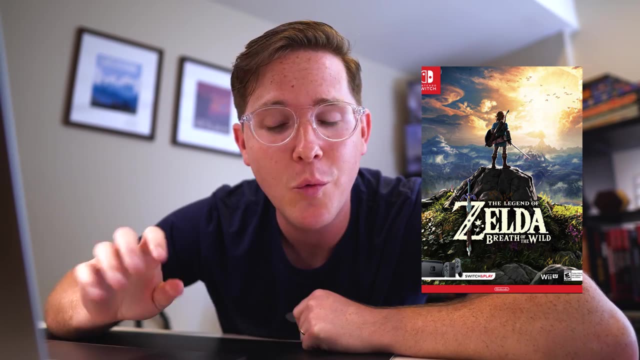 with a gypsy in my game, But I do think it would be awesome for my game to capture a similar delightfulness of adventure that The Legend of Zelda, Breath of the Wild, has in its game, when you decide to climb to the top of a mountain. 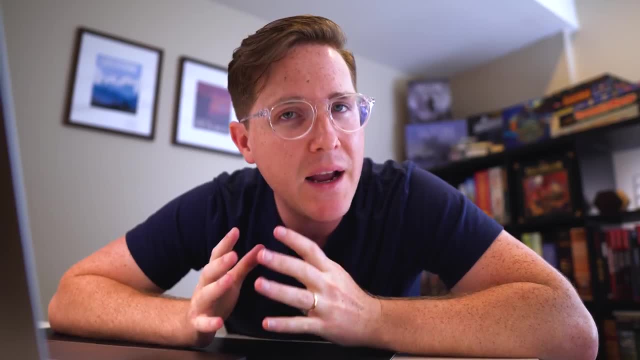 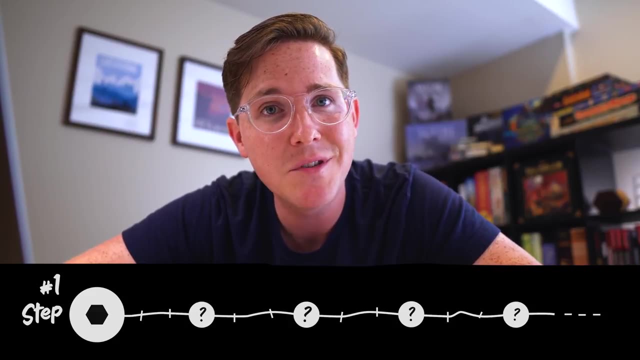 just to see what's there In my game. I've completed step one, I've thrown a decent amount of blank hex tiles on a board and now I just need to complete steps two through a hundred to find that great game that's in my head. And if I'm able to do that, then I'm going to be able to do that, And if I'm able to do that, then I'm going to be able to do that, And if I'm able to do that, then I'm going to be able to do that. 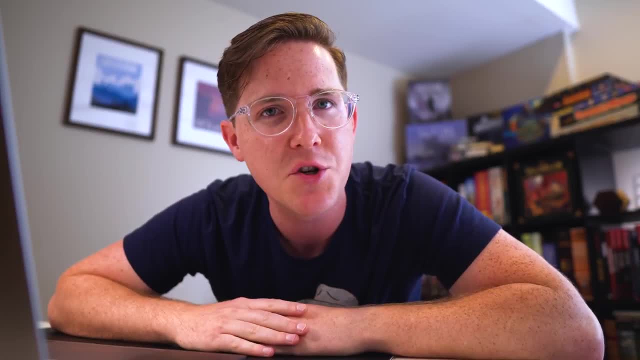 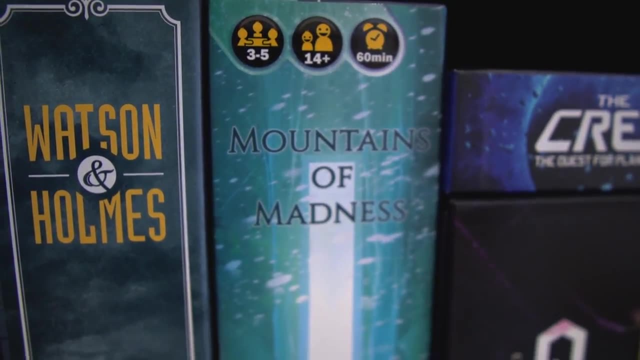 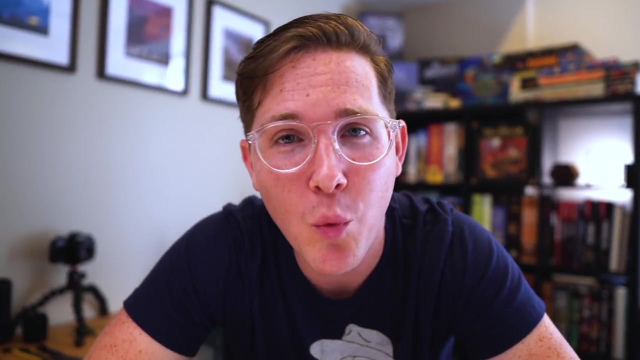 And if I'm aiming to give my players fun things to do in this hex tile exploration game, then I'd better start focusing on what's going to be on those hex tiles. I have to start by shouting out one of my subscribers who had one of the best pieces of advice about hex tiles. 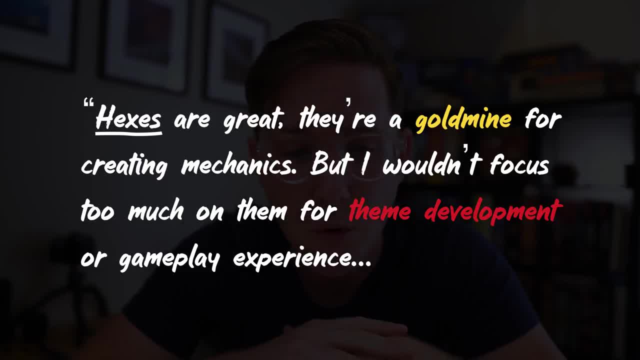 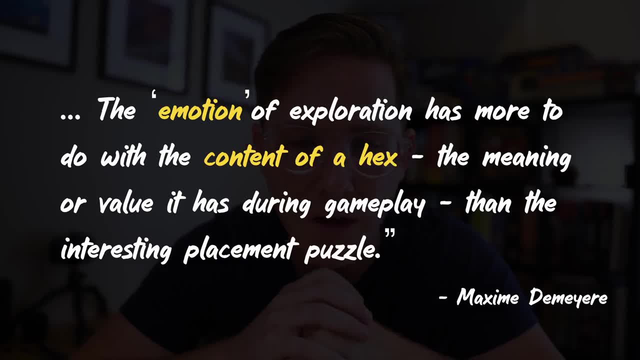 in my last video They said hexes are great, They're a goldmine for creating mechanics, But I wouldn't focus too much on them or theme development or gameplay experience. The emotion of exploration has more to do with the content of a hex. 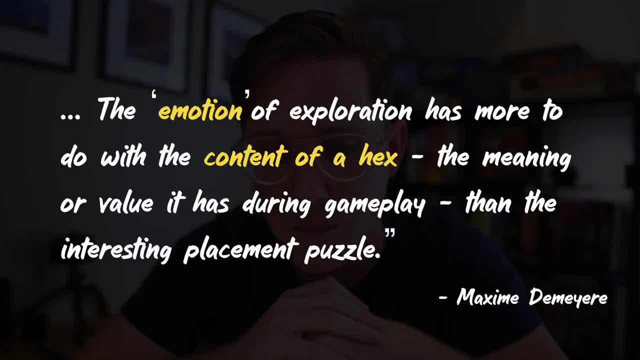 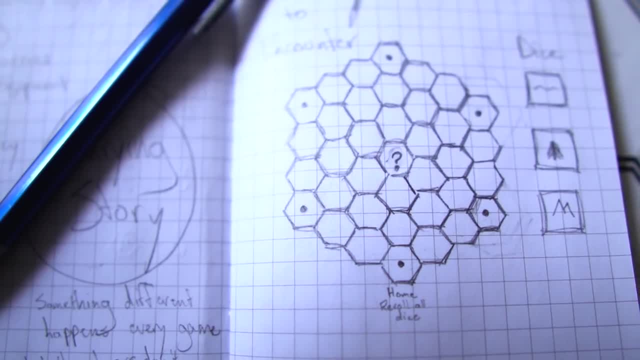 the meaning or value it has during gameplay than the interesting placement puzzle. Wow, this is awesome advice, Although I don't think that I was letting my hex tiles inform too much of the theme for this game. when I read that comment, I took a step back. 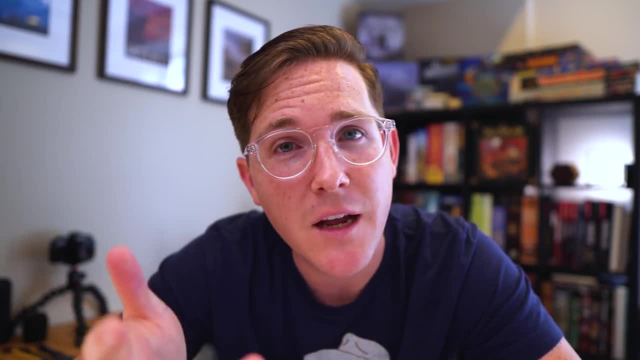 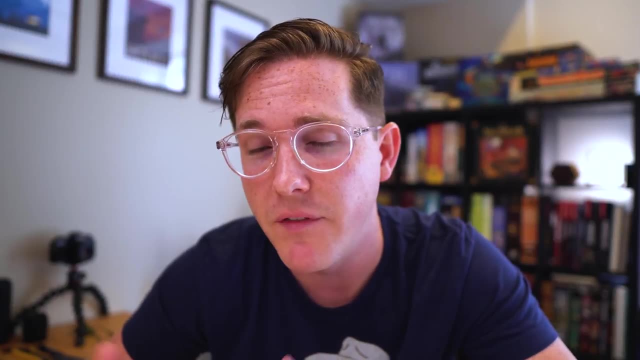 to make sure I wasn't heading in that direction with my design. I simply want the hex tiles to add to the sense of exploration. whenever you move on to an unoccupied space and end up flipping a tile to reveal the available actions on that space. 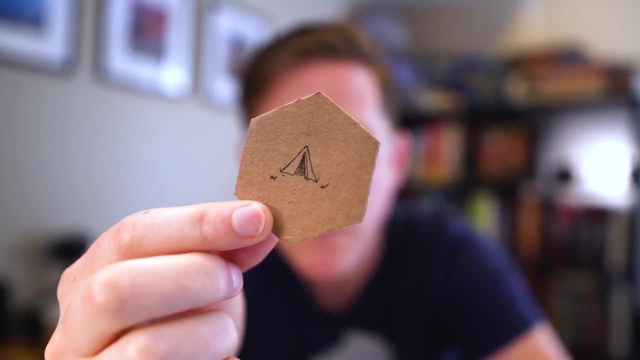 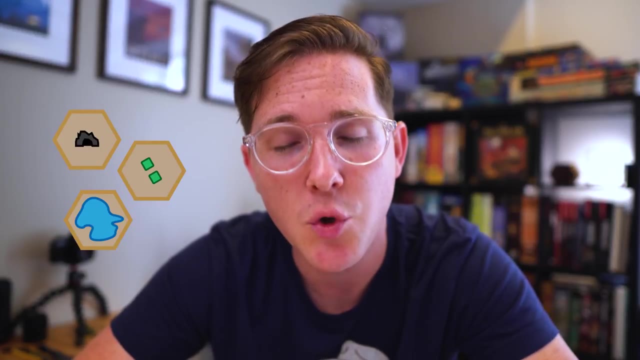 These tiles will likely be small and will only be able to deliver minimal terrain textures and maybe one or two icons at a time. When a player reveals and lays down a tile, I want them to immediately identify what's on the tile and what they can do on it. 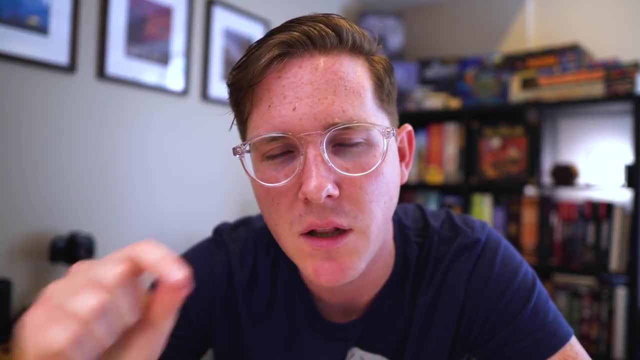 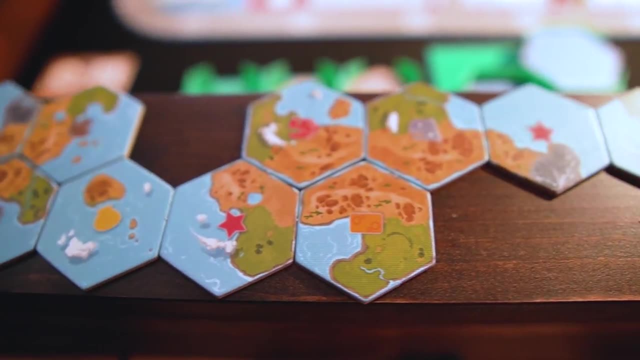 Although it's tempting to give hex tiles a lot of power by putting a lot of information on them, I think it would be bad design for the size of these tiles, Similar to tapestry. I want the iconography on each hex tile to be very minimal. 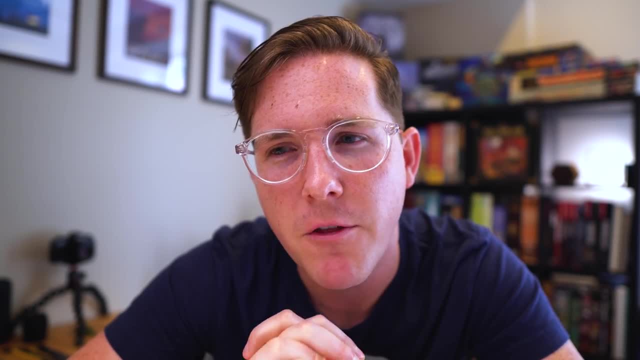 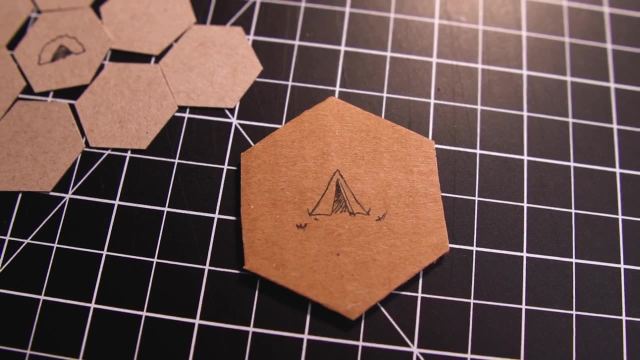 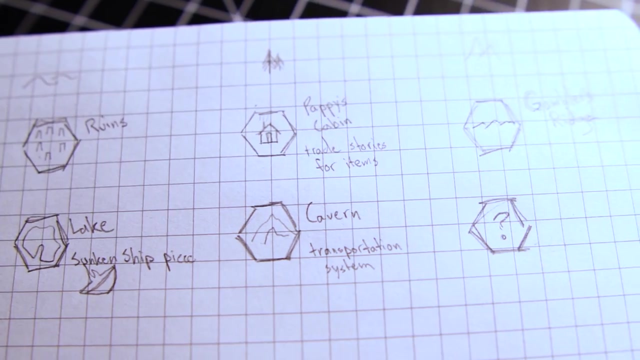 However, I don't think that that means that they can't be used to deliver the theme in a meaningful and effective way. Let's say, we want to add special locations in this exploration game that allow players to take unique actions on them when they're occupying those spaces. 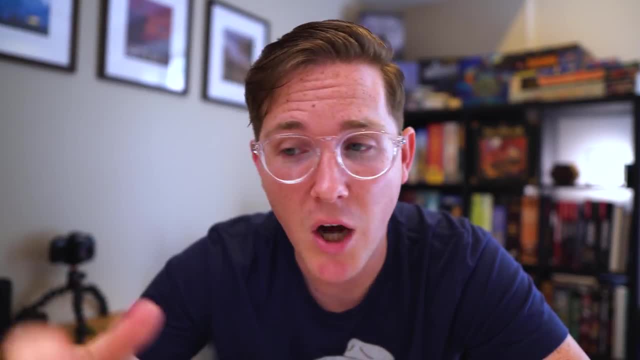 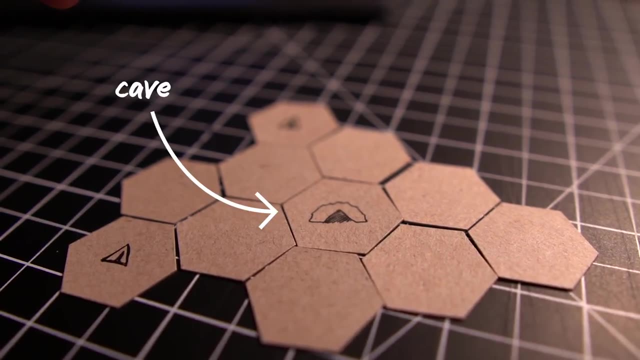 Pretty simple, right? Let's say a player explores a space in the forest, uncovering a tile and revealing the entrance to a cave. I could add a simple icon on that tile representing the mouth of the cave, And players all around the table can immediately. 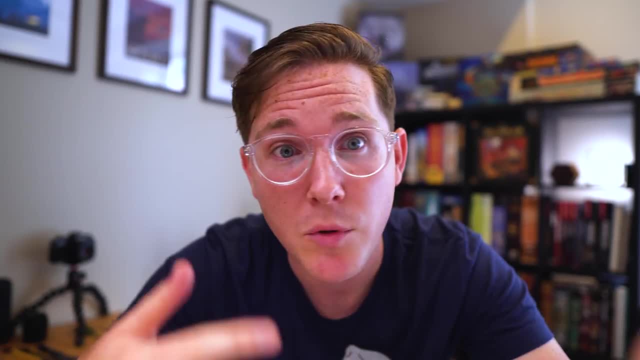 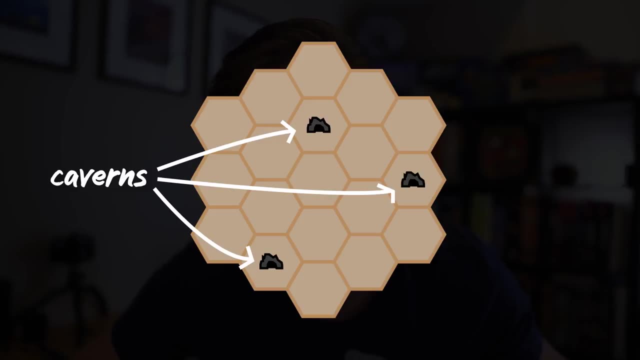 identify that that's a place where they can enter the cave and spend multiple turns discovering what's inside, taking risks and finding rewards. What if I wanted a system of caverns connecting throughout the board And, as a player, when you entered one cave entrance? 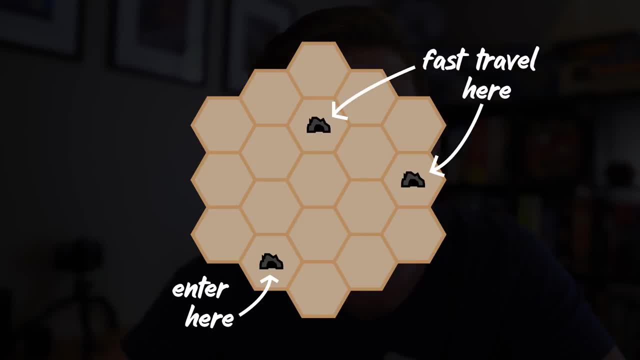 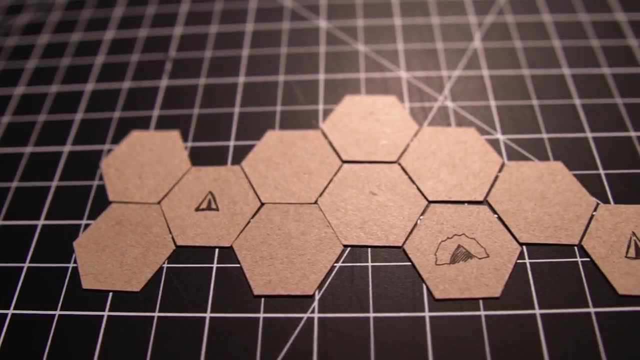 on a turn, you know, on your next turn you can fast travel to any other cave entrance on the board. I could also do something cool with campsite locations that are also unique. understandably, in the mountains or forest You may come across an abandoned campsite. 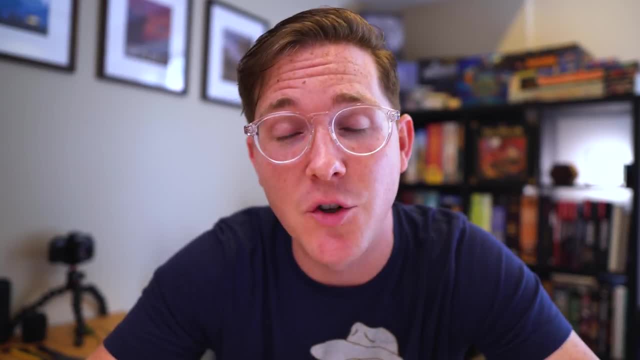 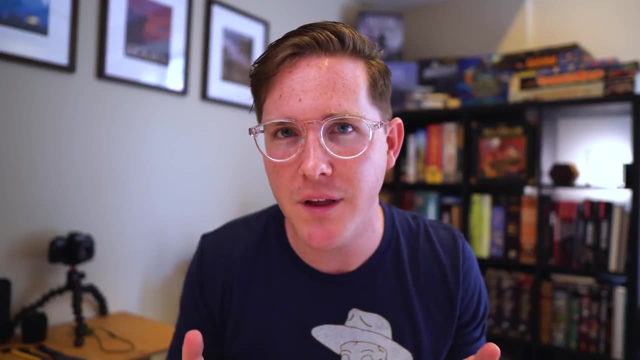 that allows you to perform rare actions that are available when you decide to rest there As a player. you may be absolutely relieved when you see a campsite tile, because you know you've been without a proper place to sleep and rest for days or turns. 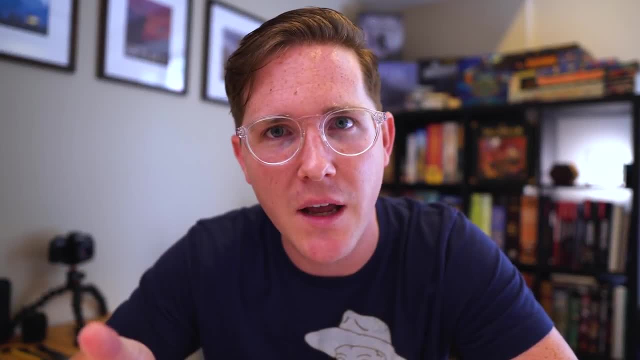 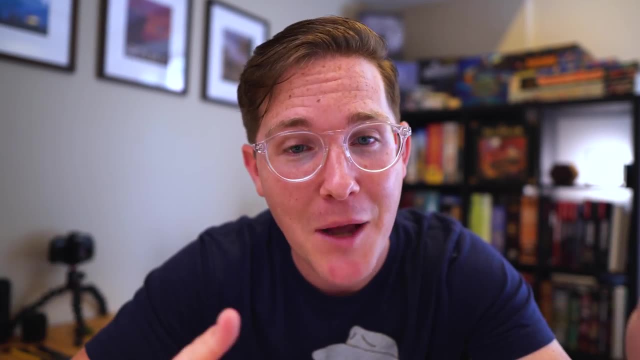 And you desperately need to cash in some of the cards or tokens that you have in your hand, because they've been dead weight in your hand this whole time until now. See, You see how even the rough shape of a triangle, a campsite, 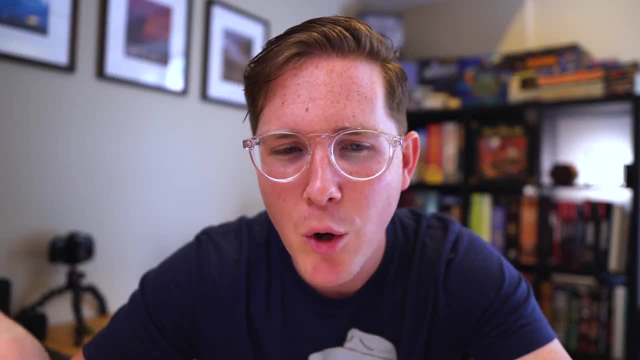 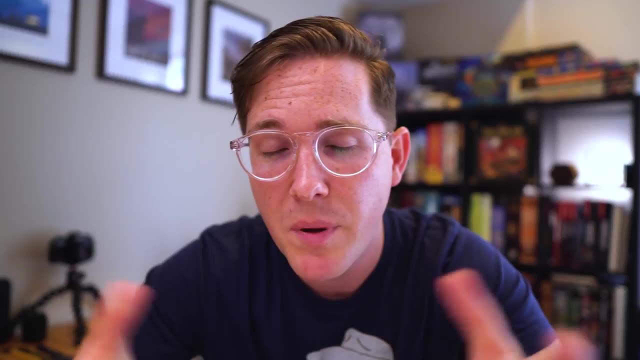 could represent So much to a player in the game. The hex tile may only show a minimal terrain type and then a single icon on it, But those two things could mean a variety of things in your game, depending on the possibilities that you tie into them. 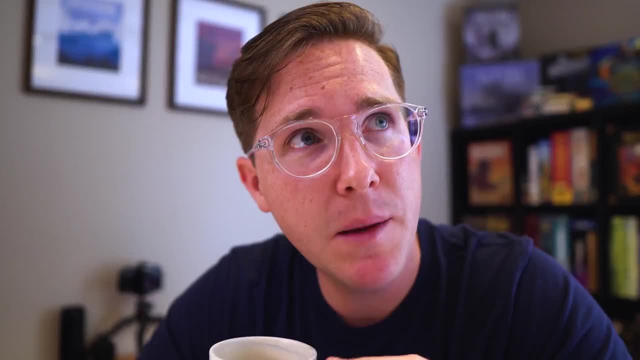 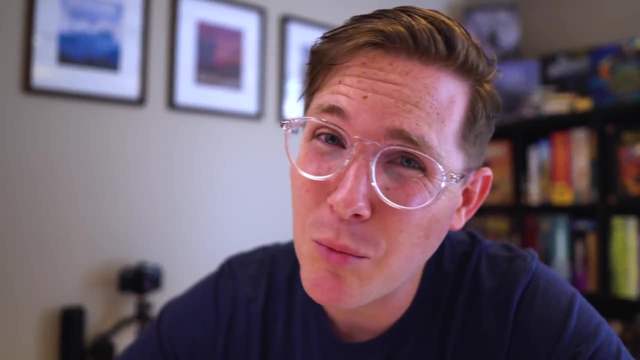 OK, let's stop talking about hex tiles, Let's talk about something else. Let me show you the nighttime dice For me. I'm not opposed to using dice in a game. I actually really like dice. A game really doesn't feel like a board game. 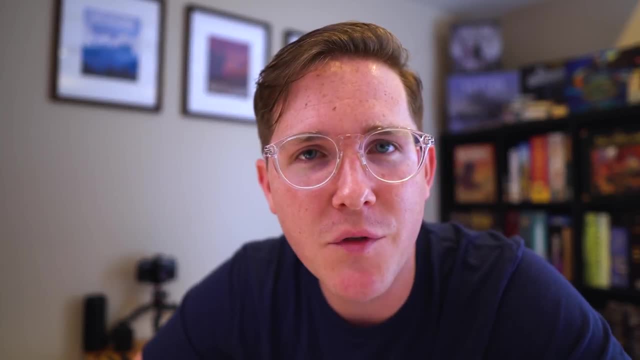 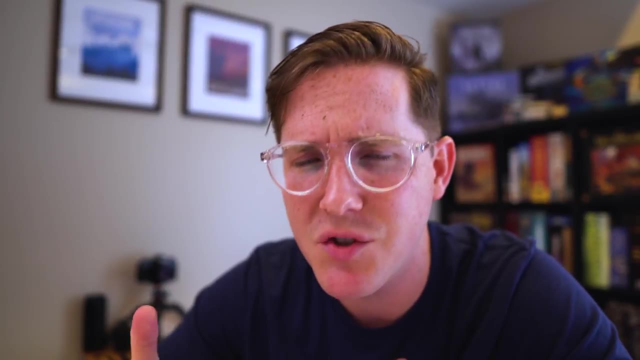 if it doesn't have dice in it, Hot take. However, I understand for some designers it could be a turn off depending on the level of chance or luck that it adds to the game. For the role dice could play in my game, I think it's just fine. 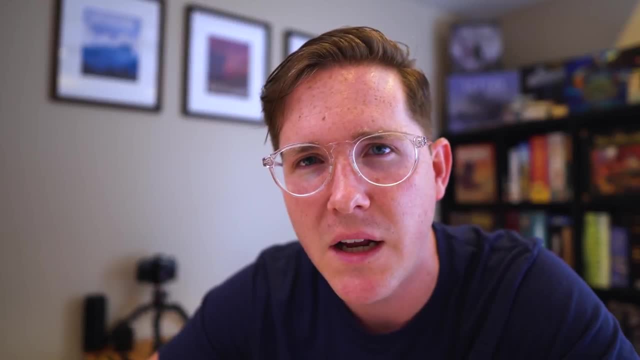 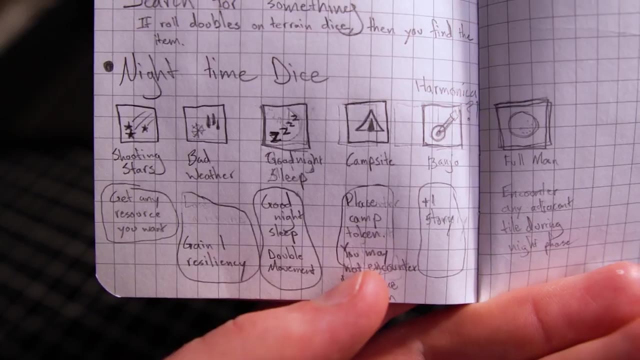 Because the dice mechanics in my game shouldn't unfairly disadvantage or advantage some players And shouldn't make a huge difference in when someone wins. I have this loose idea of having a nighttime fate That is also played with a dice, with a single dice roll. 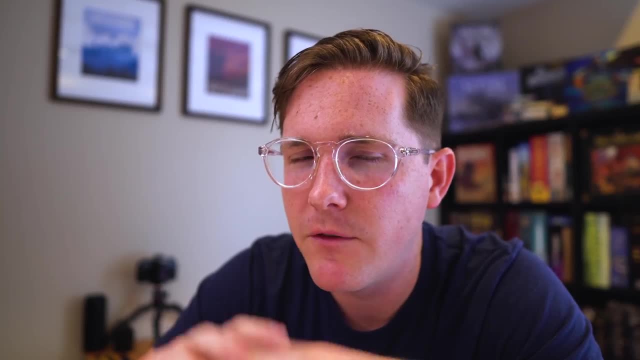 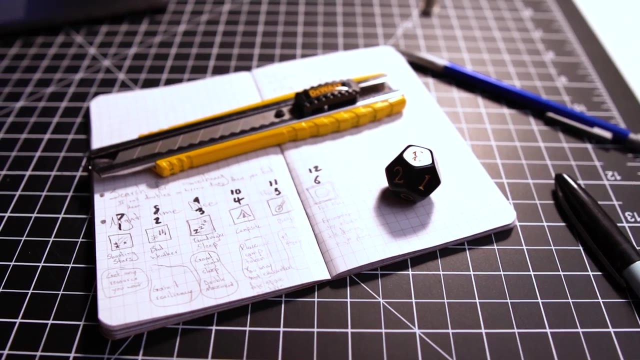 It would be a brief phase where players know that a full day has come to a close And their movement and adventure are restricted to the darkness of nighttime. During the nighttime phase, one player rolls the nighttime dice And the result quickly determines what. 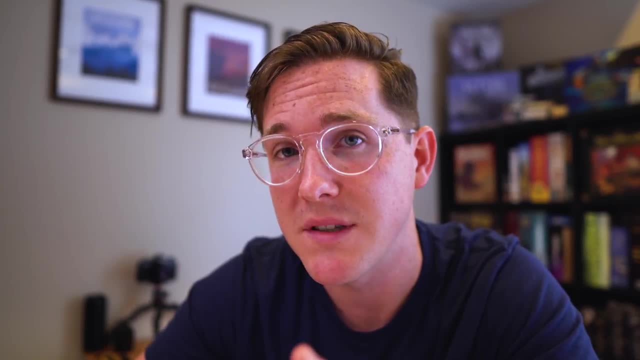 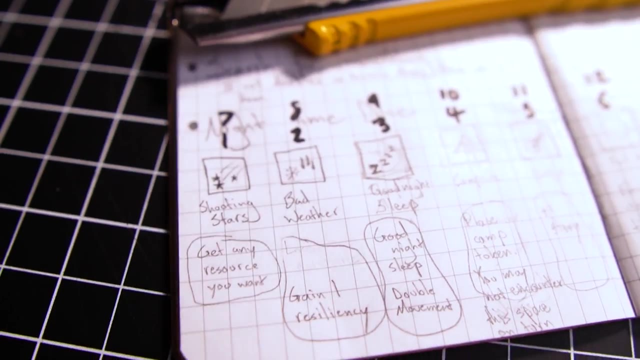 happens in that nighttime phase and also what benefits the players receive. The night could bring an inspiring night sky with a few shooting stars, and that allows players to make a wish and get one of any resource they choose, Or the night could bring bad weather. 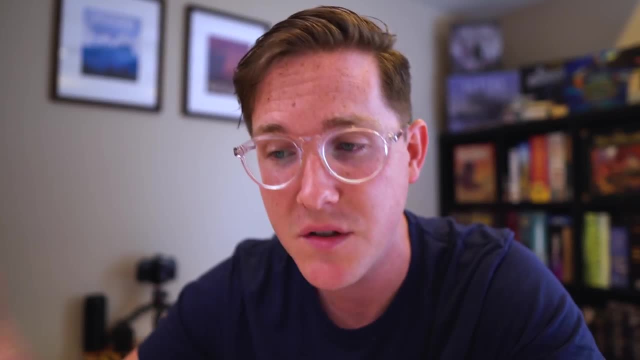 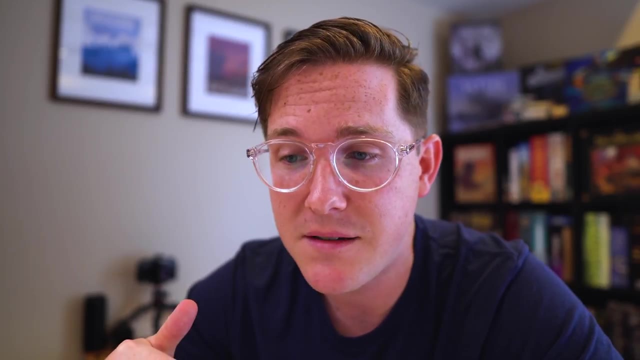 and the players are forced to endure a downpour of rain or snow in which each player gains a resiliency point, actually benefiting them in future turns. Or maybe you roll the dice and it says that the players all get a great night's sleep. And they're allowed to take double movement on their next turn. Maybe you roll the dice and it has a full moon on it And that full moon casts enough ambient light throughout the night that players can actually take an extra exploration turn during the night phase. 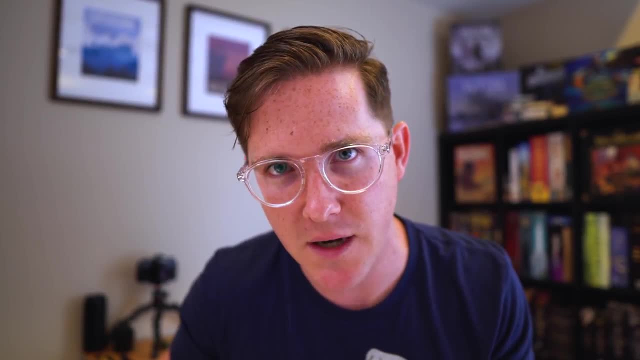 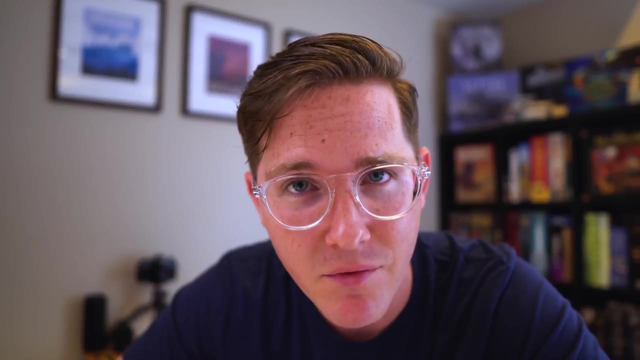 extending that phase and making it a little bit more opportunistic during night. This is one idea I have for introducing dice in the game. Yes, the results are random each nighttime phase, But at least they're thematic and all players gain the same benefit. 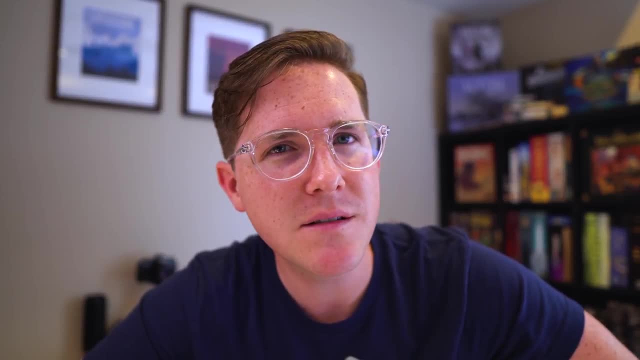 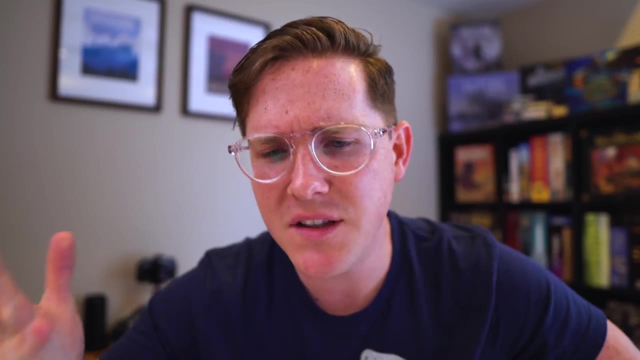 I kind of like that idea. As a designer, if I don't find reasons to introduce disadvantages to specific players in order to balance the game out, then why should I? Why can't I just let my players have fun and see some darn shooting stars? 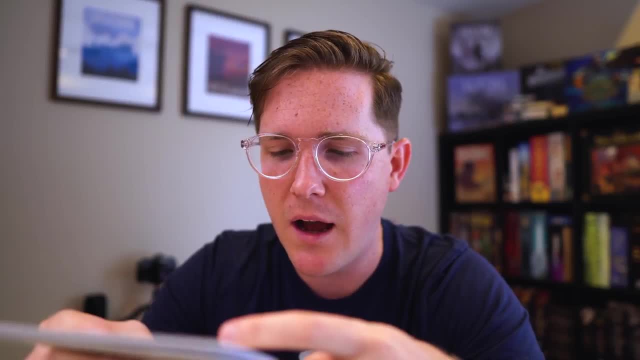 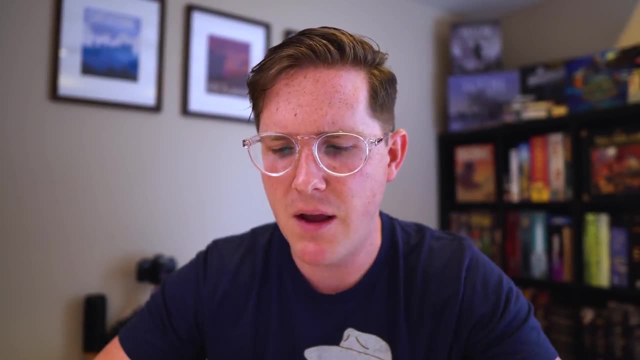 The last thing I'm going to share today is about the winning conditions. I think to really honor this theme of a personal journey that you're making out in the wilderness as a player, and the reason why you're out there in the first place is that it's something personal to you. 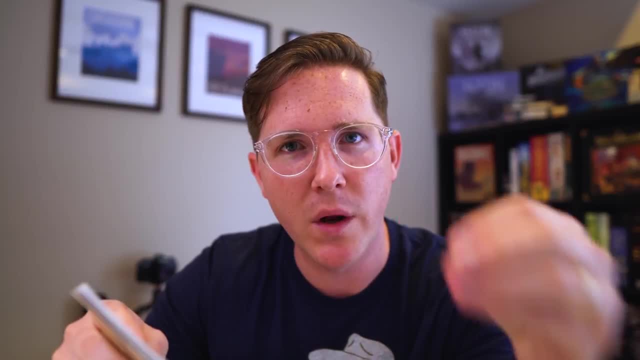 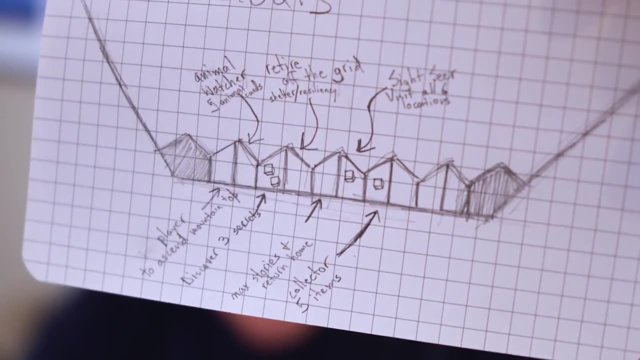 You have a personal goal. What if players were able to pick the winning conditions at the beginning of the game? Players could literally choose what they want to accomplish in the game. The goals could be thematic as well, And also these goals may not be competitive. 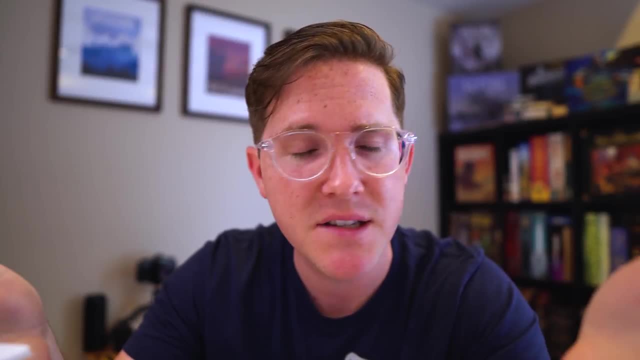 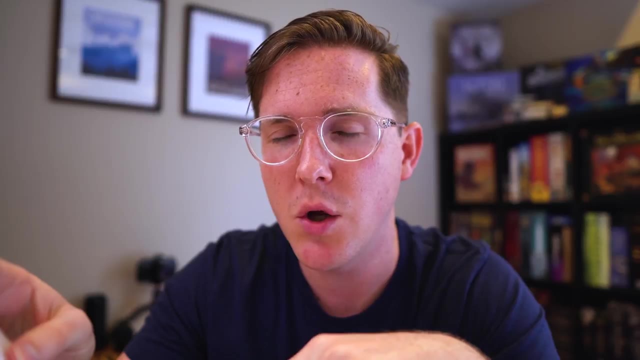 or first come, first serve. So two or more players could have the same goal And if they achieve it throughout the game they both get to check that off of their list. But maybe the winning player is the one who accomplishes all of their goals first. 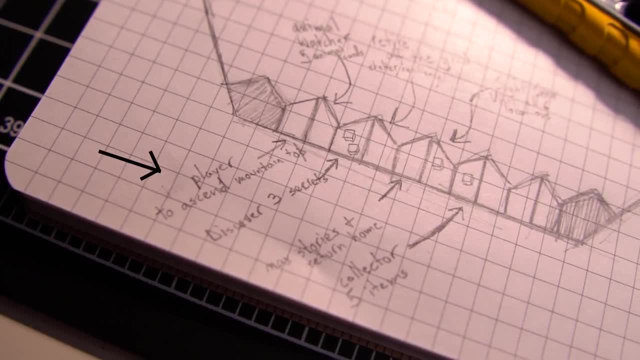 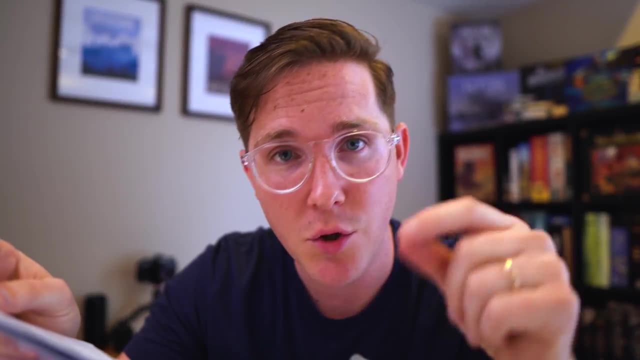 As a player. maybe you decide to try to ascend to the top of the mountain, And once you do that- which it may be quite difficult to do, especially early in the game, But once you do that, then you've achieved that goal. 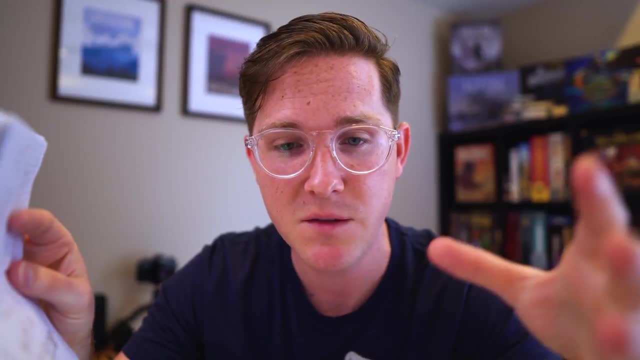 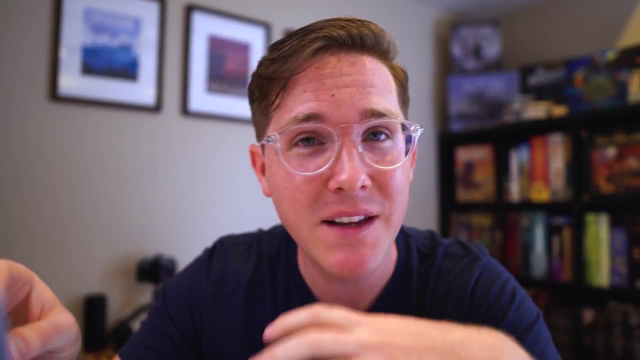 and you check it off of your list, You place a star or you pick up a token or something visible that's public to the rest of the players, that they know that you've completed one of your goals And maybe you're the next player to look out for. 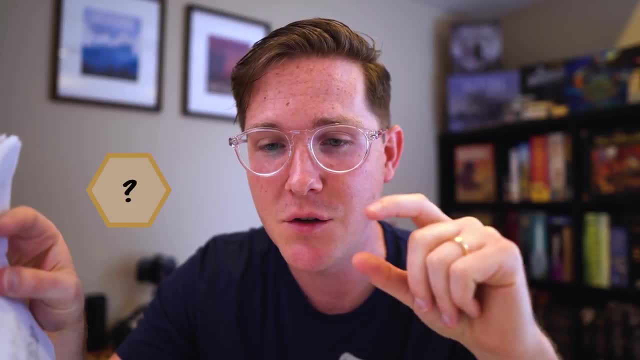 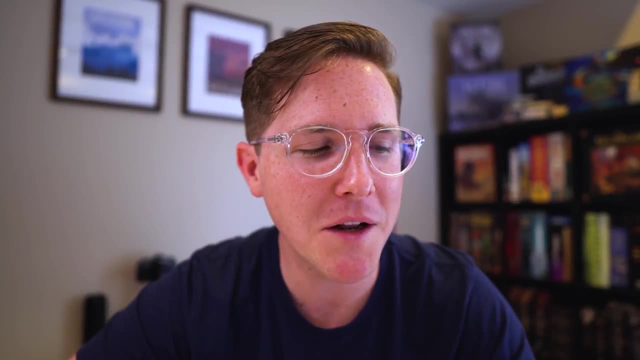 Maybe on all of these tiles there's specific tiles that have secrets on it, And you're wanting to be a player that finds at least three secrets And once you do, then you complete your goal. This is kind of a funny one, but what if your goal is literally? 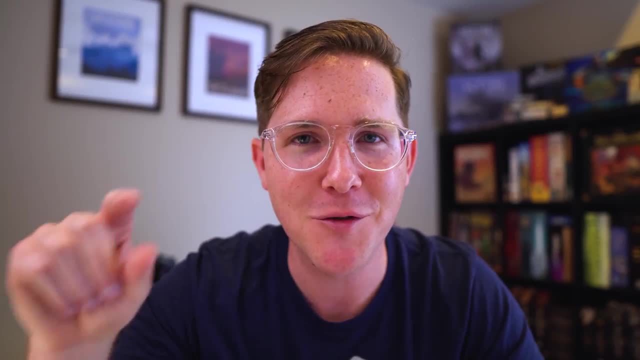 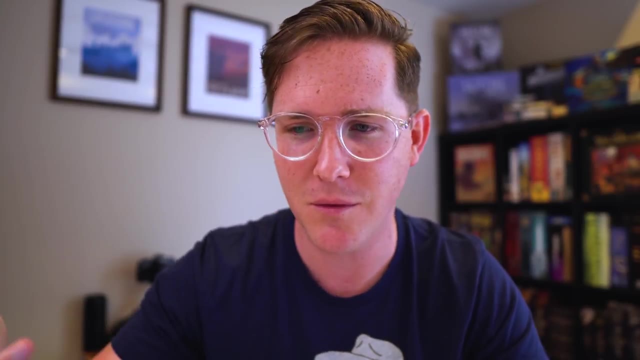 to retire out in the woods. You want to find one of those campsites and there's a special card or an action that you take after you've accumulated other tokens or various things that allow you to end your game and finish that way. It's thematic because you would literally 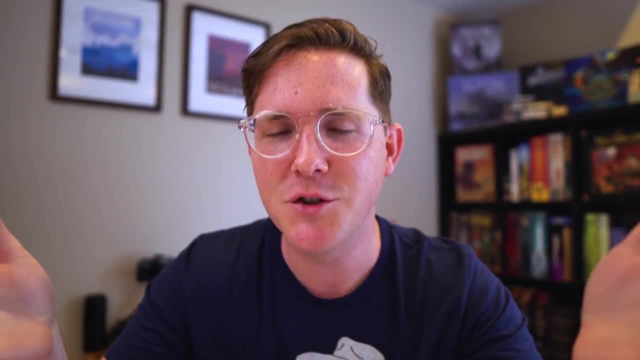 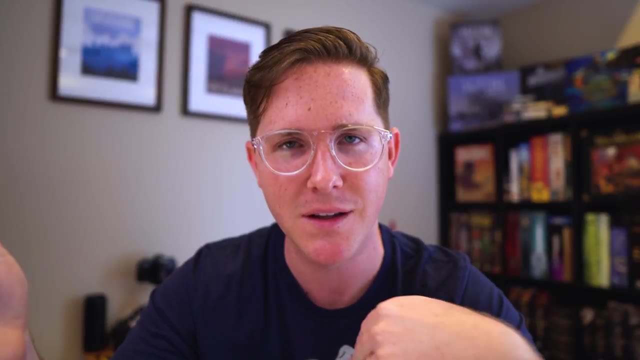 imagine yourself just living out there from that point on, And maybe the general story of all the characters is that they're going out into this wilderness to eventually come back to civilization or go back home, But you're the lone person who's going to stay out in the woods forever. 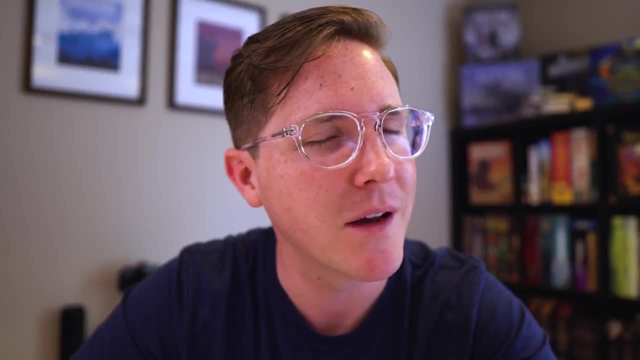 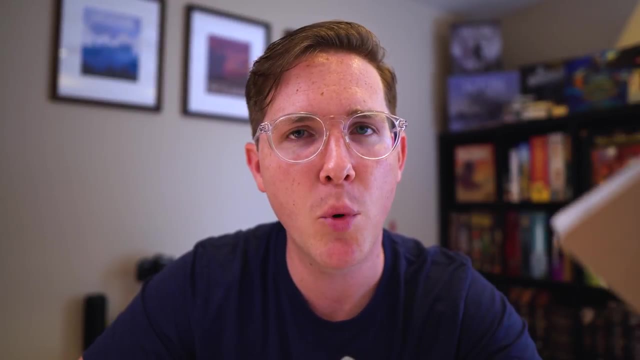 Obviously there would be conditions that you would have to meet to do that, but I think that would be kind of fun. And what if on the cards, like, there are special cards for sightseeing or depending on the weather that day or that morning? 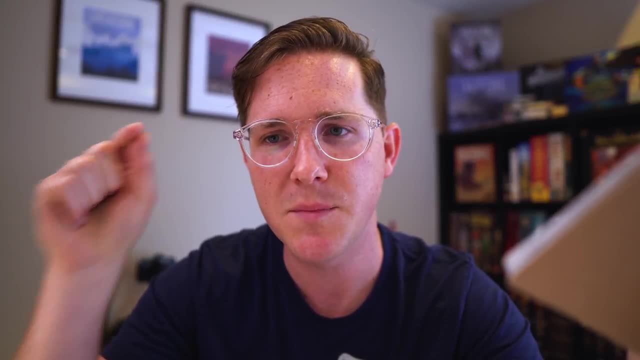 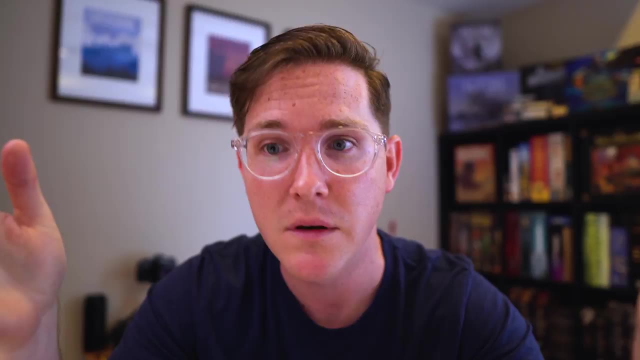 if you're able to play a specific card on your turn or be in a special spot, you're able to see the top of the mountain or the clouds part, and you're able to see the glistening snow at the very top of the mountain. 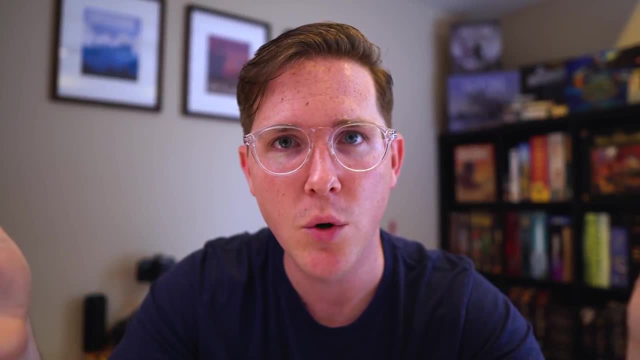 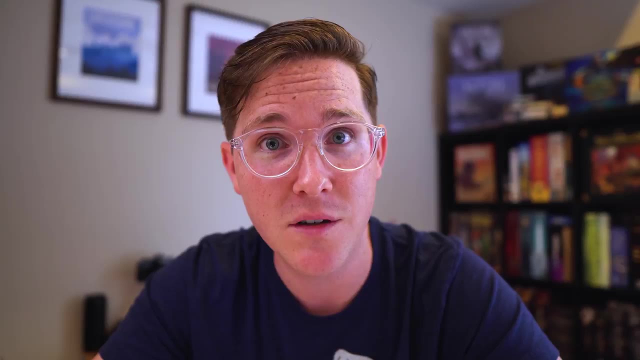 And that is in itself a sightseeing goal for you. So if you see enough sights and you play enough of those special sightseeing cards, and that too could be a winning condition. Those are just examples. I really like the idea of even the winning conditions. 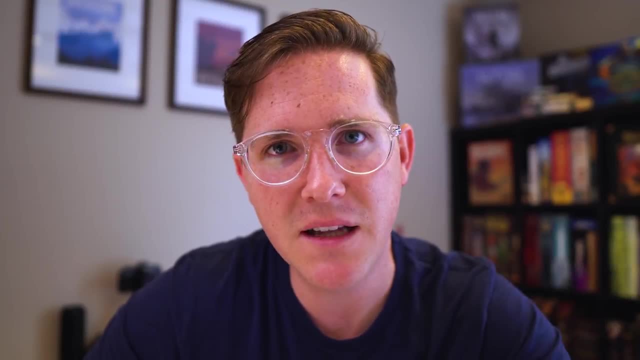 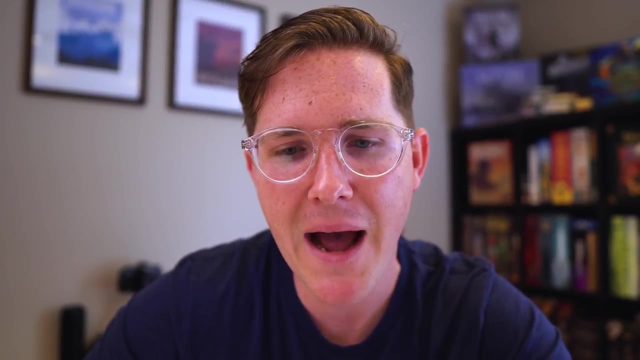 being thematic, where, if you accomplish something that makes sense in the universe of your board game, like this when you're exploring a mountain range or a forest- the goals that you accomplish match what you imagine a person would want to do out there by themselves. 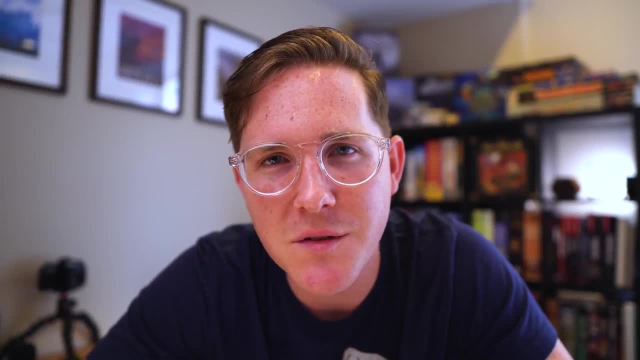 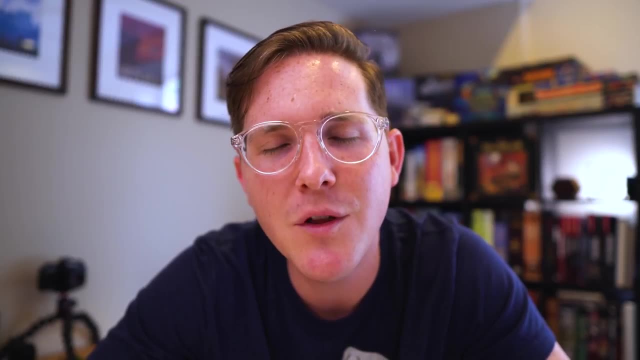 That's all I have for today. Once again, thank you so much for the support. so far, I've passed 100 subscribers, which is amazing. You guys may not realize how incredible even those small milestones may make me feel, so thank you. 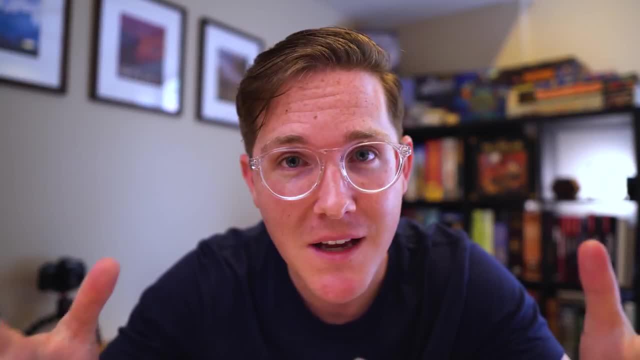 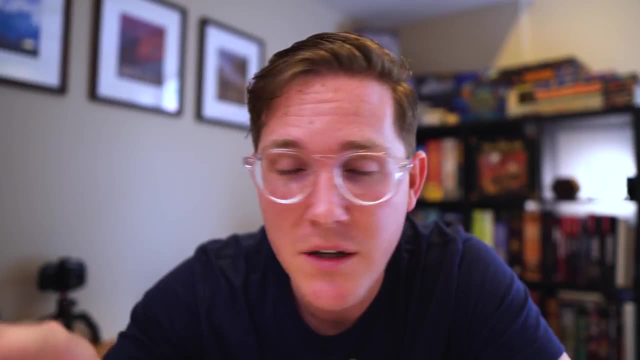 OK. so like I said in my previous video- and I'm going to keep saying it- please share your own ideas for board game designs. So if you are creating a game right now, share some comments down below to let everyone else know what you're designing. 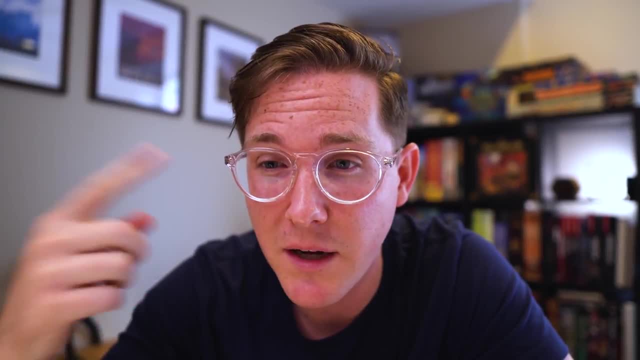 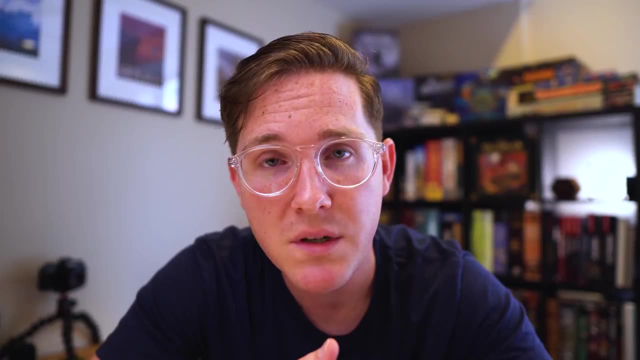 One, because it helps me learn from your ideas and also just sparks my creativity in terms of thinking about multiple mechanics that I might want to integrate into my own games And separate from sharing your own design ideas. let me know how else I can be plugged. 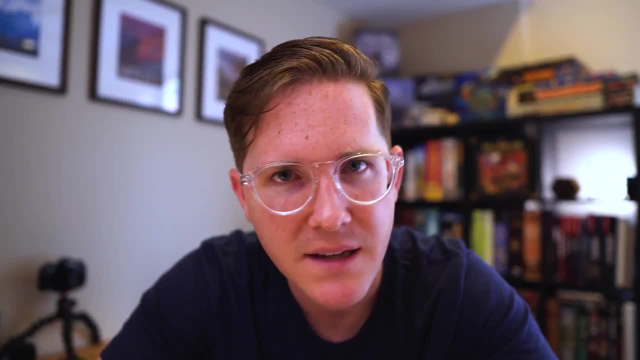 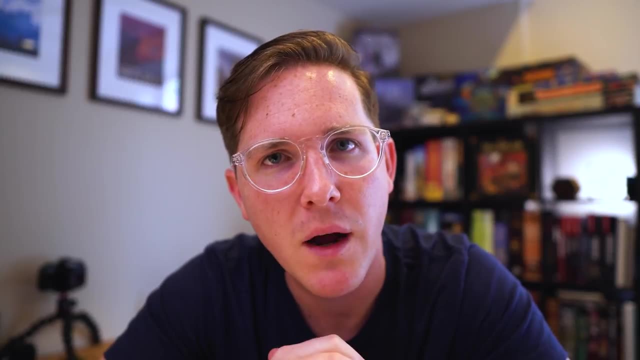 into this community of board game design. I know that there's podcasts that I'm listening to and other people on YouTube, but share those people in those communities with me so I can stay plugged in in the right way. Thank you so much for watching and I 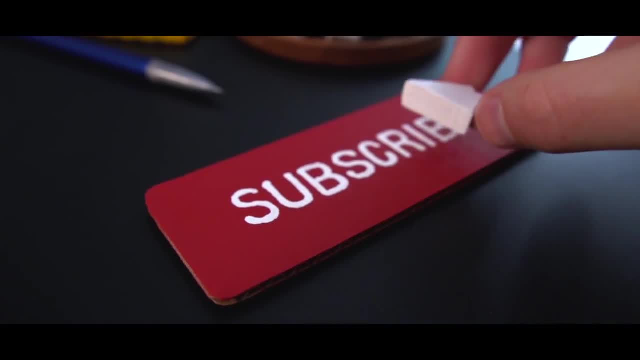 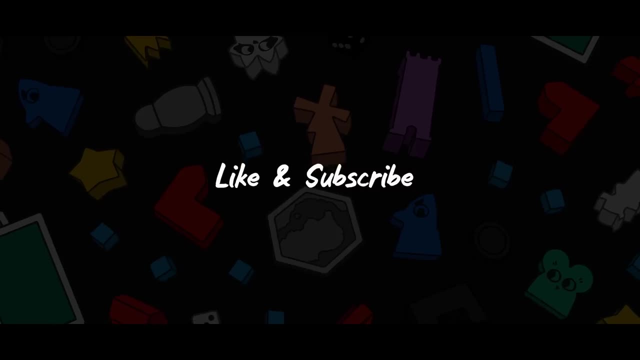 hope you have a great day. I'll see you in the next video. 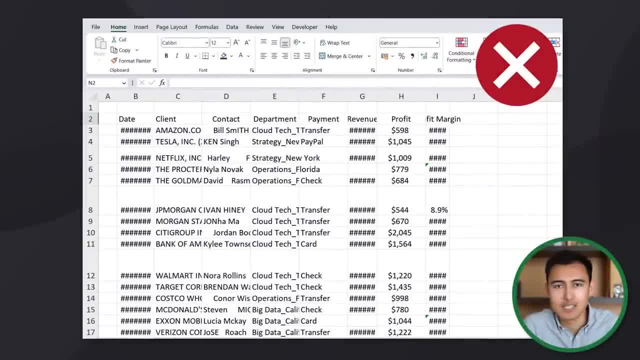 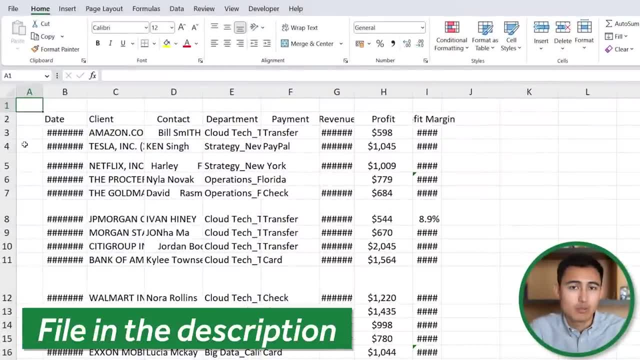 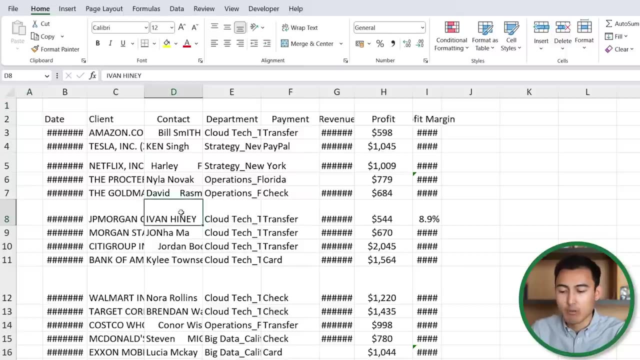 In this video we'll go from having a raw data set like this to converting it into a clean excel file in just 10 steps. so let's get into it and you can download this exact same excel file in the video description for free. so over here you can see that we have the data set. this is the raw one, basically. 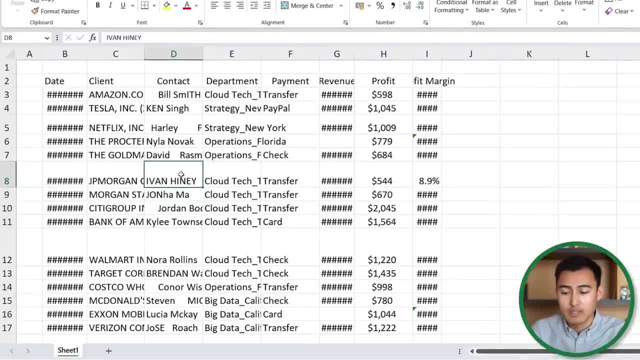 but before we make any changes to it we should probably save a copy. so you can either save a new excel file or just save this sheet by clicking the control key and just dragging that sheet. so you have two separate ones. all right, now we can get started with step 1 out of 10, and first you 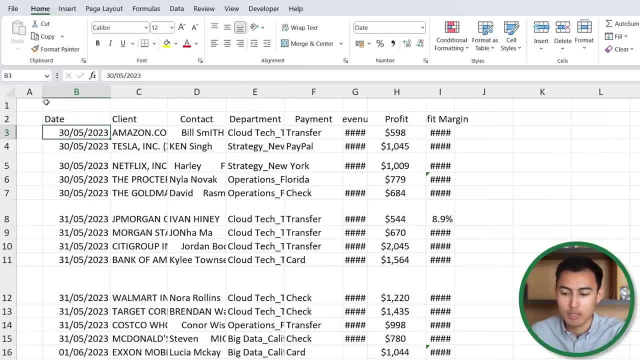 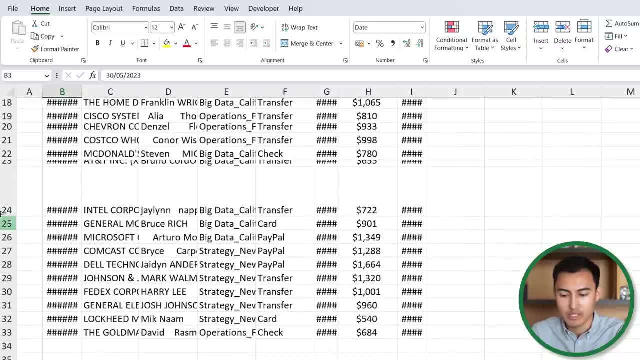 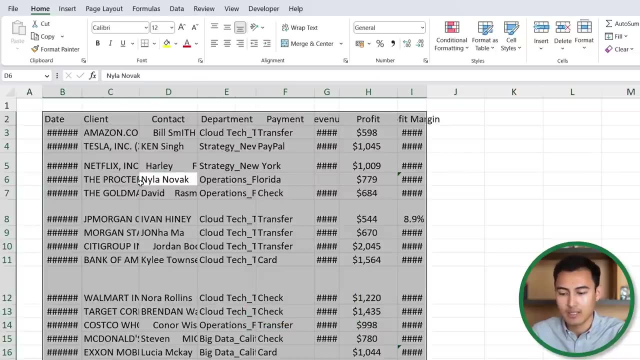 can see here that these columns are just too short. if i stretch them out, the number looks okay, but if i close it down, you get this sign over here. same thing with the rows. some rows are just too long, like this one right over here, so let's go ahead and refit this by just going to ctrl a, that's. 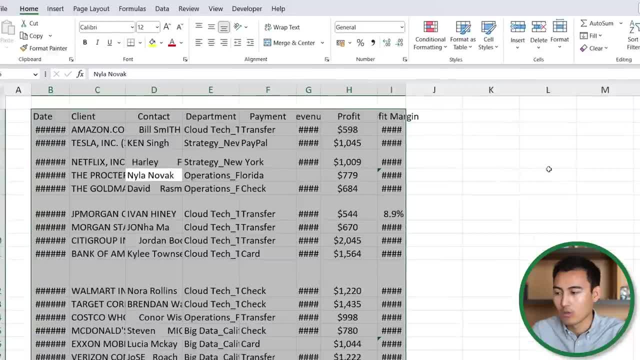 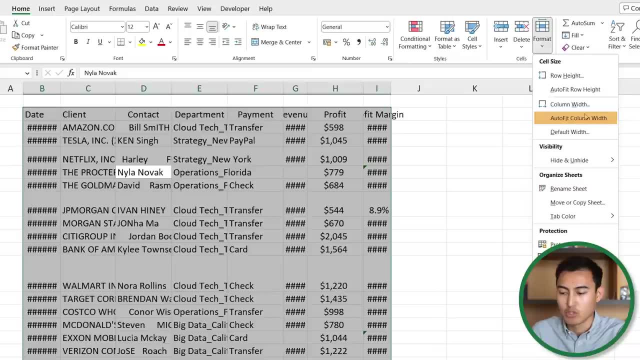 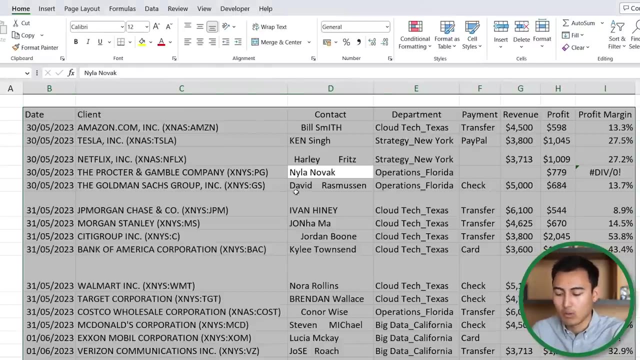 going to select the entire table for us, and then we'll go over to the side where it says format and you can auto fit the row width and the column width. now the shortcut for these is just alt h o i, that's going to auto fit the columns, and then alt h o a to auto fit the rows. now you can see that we.